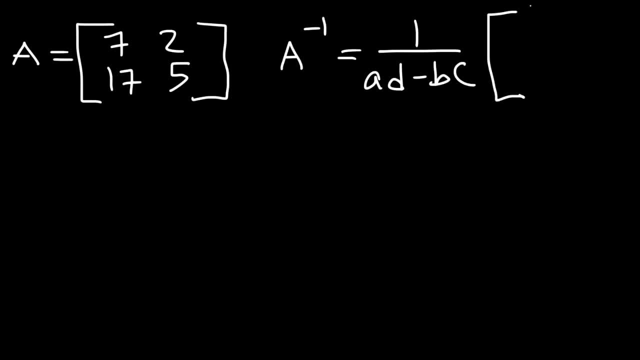 minus BC times the matrix with the following elements: D, negative, B, negative C and A. Now matrix A contains the elements A, B, C, D, in that order. So using that, go ahead and find the inverse of matrix A. So if we match up the letters we can see that. 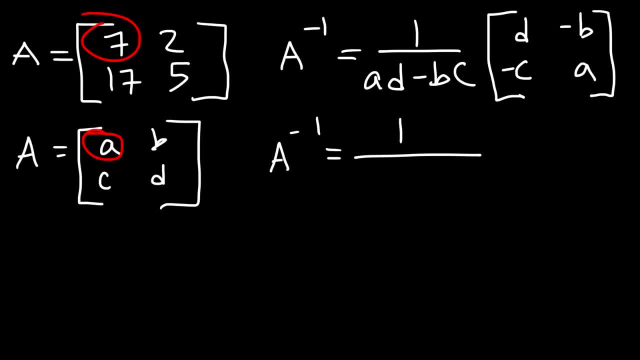 A is 7.. So let's replace A with 7.. D is equal to 5,, B is 2, and C is 17.. Now D is still 5, negative B, that's going to be negative 2, negative C is negative 17,. and. 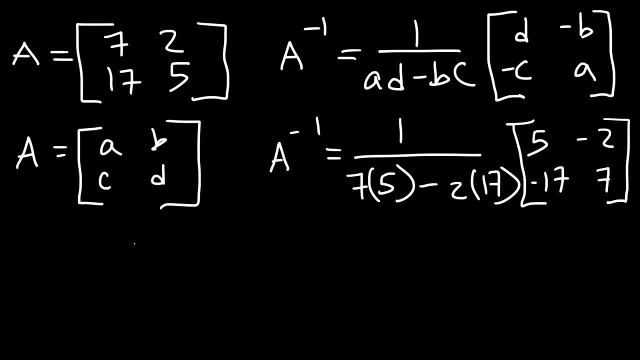 A is 7.. So let's replace A with 7.. Now D is equal to 5, B is 2, and C is 17.. Now A is 7.. 7 times 5 is 35.. 2 times 17 is 34.. And then 35 minus 34 is 1.. So this whole. 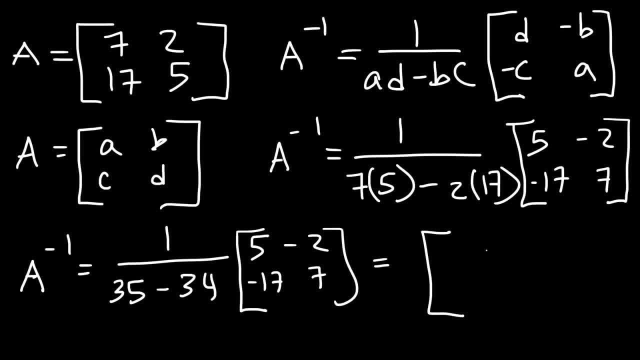 thing is 1 over 1.. So the inverse of matrix A is simply 5.. Negative 2, negative 17, and 17.. So that's a quick and simple way to determine the inverse of a 2 by 2 matrix. Now how can we confirm that this is indeed the inverse? So here's: 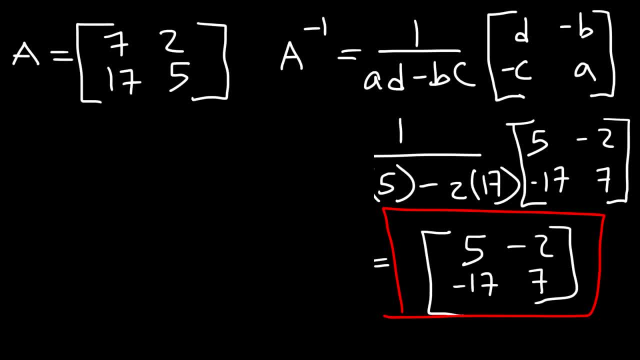 what you can do. If you take 5 and multiply it by its reciprocal 1 over 5, that will give you 1.. Now if you take matrix A and multiply it by its inverse, it will give you the identity matrix And we're dealing. 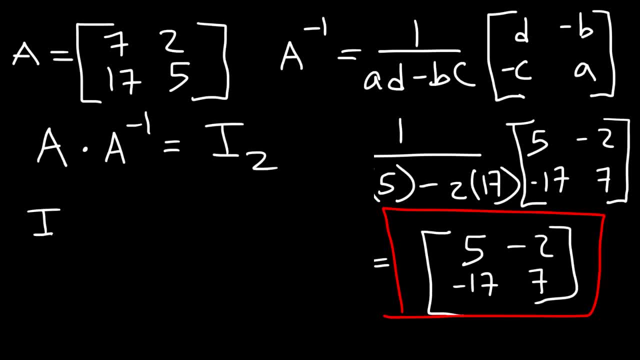 with a 2 by 2 square matrix, So we'll call it I2.. So the multiplicative identity matrix looks like this. It's So the main diagonal contains ones. So if we multiply A by the inverse of A, our answer should look like that: And if we get that, then that tells: 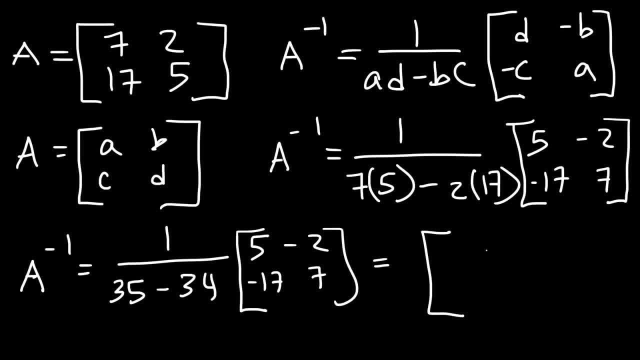 thing is 1 over 1.. So the inverse of matrix A is simply 5.. Negative 2, negative 17, and 17.. So that's a quick and simple way to determine the inverse of a 2 by 2 matrix. Now how can we confirm that this is indeed the inverse? So here's: 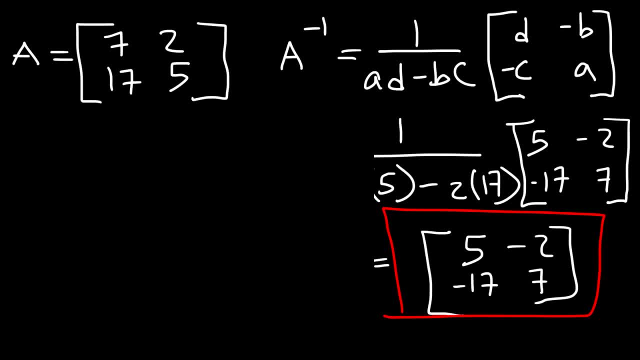 what you can do. If you take 5 and multiply it by its reciprocal 1 over 5, that will give you 1.. Now if you take matrix A and multiply it by its inverse, it will give you the identity matrix And we're dealing. 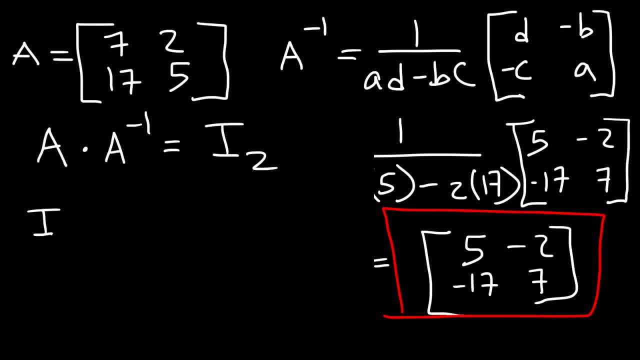 with a 2 by 2 square matrix, So we'll call it I2.. So the multiplicative identity matrix looks like this: It's 1, 0, 0, 1.. So the main diagonal contains 1s. So if we multiply, 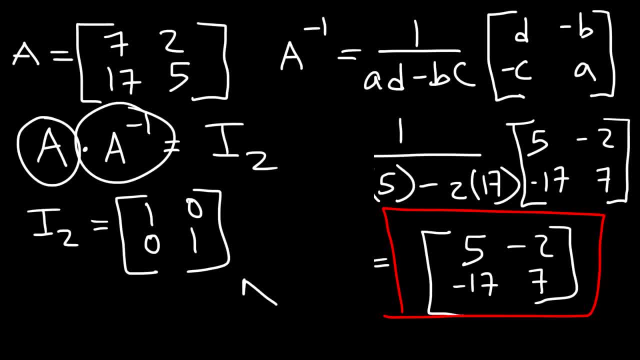 A by the inverse of A, our answer should look like that: If we get that, then that tells us that it's 1.. So if we multiply A by the inverse of A, our answer should look like that: If we get that, then that tells us that it's 1.. So if we multiply A by the inverse, 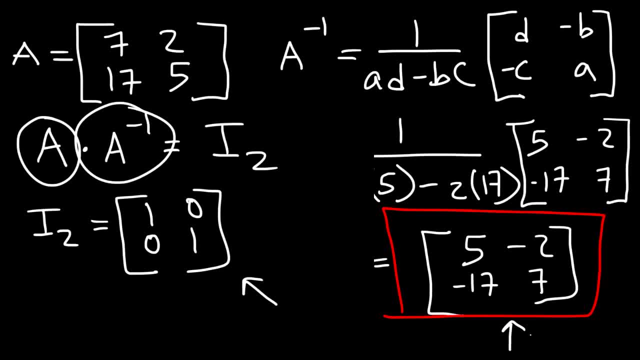 of A. our answer should look like that: If we get that, then that tells us that it's 1.. So this is indeed the multiplicative inverse of A. So let's go ahead and multiply matrix A with the inverse of matrix A. 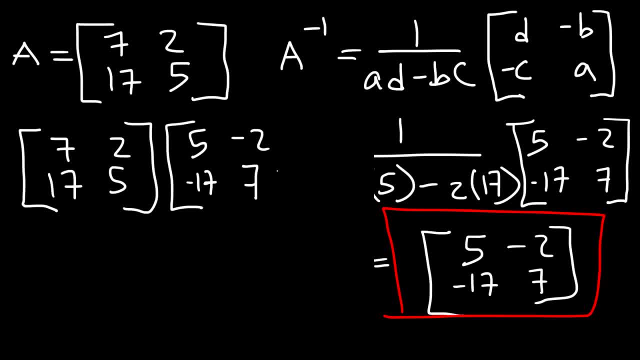 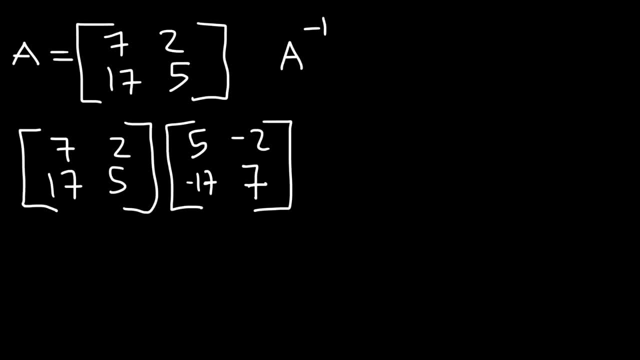 And let's see what we get. So we need to multiply the elements in row one by the elements in column one and add their products And we're going to place that answer in the first row, first column. So it's going to be seven times five plus two times negative seventeen. us that it's 1 over 1.. So it's a 1 over 1.. And it's going to be 2 over 1.. And then if you take matrix C and multiply it by its inverse, it will give you 1 over 1.. So if we 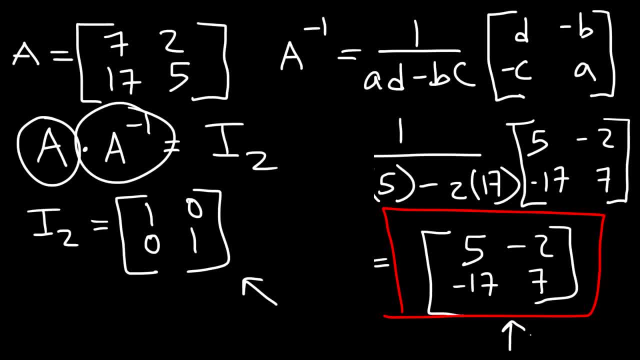 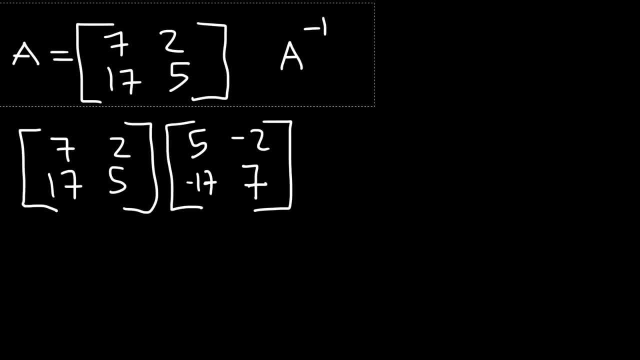 that this is indeed the multiplicative inverse of A. So let's go ahead and multiply matrix A with the inverse of matrix A And let's see what we get. So we need to multiply the elements in row 1 by the elements in column 1.. 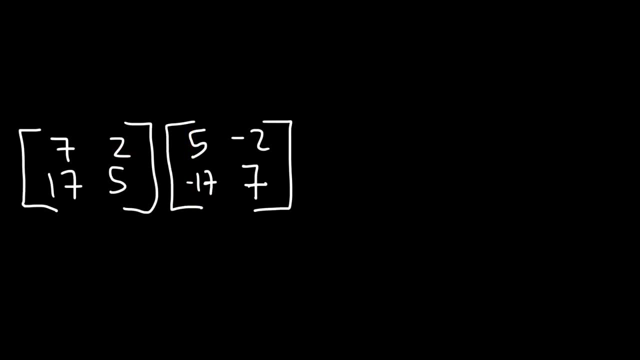 And add their products And we're going to place that answer in the first row, first column. So it's going to be 7 times 5 plus 2 times negative 17.. And then row 1 times column 2. So that's going to be 7 times negative 2 plus 2 times negative 17.. 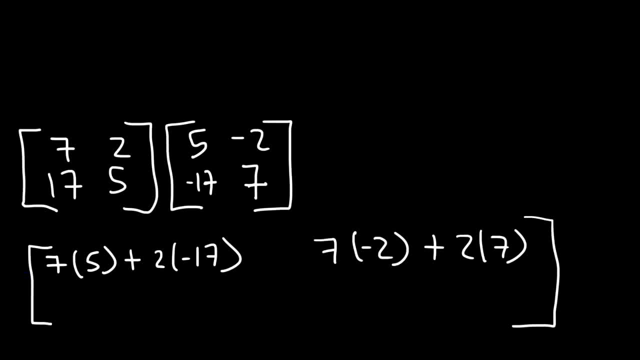 Plus 5 times 7.. And then it's going to be row 2 times column 1.. So that's 17 times 5 and 5 times negative 17.. And then, finally, row 2 times column 2.. So that's going to be 17 times negative 2 plus 5 times negative 2.. 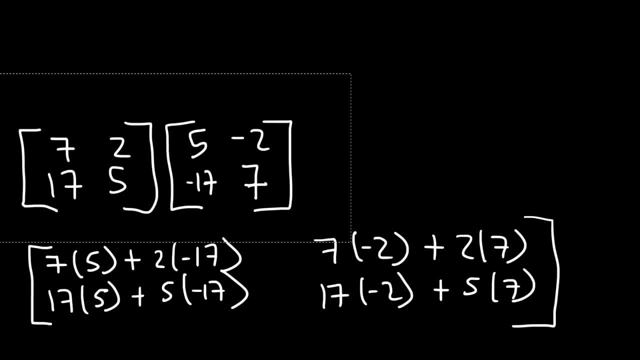 7. so now let's simplify: 7 times 5 is 35, 2 times negative: 17, that's negative 34, 7 times negative 2 is negative: 14, 2 times 7 is 14, 17 times 5 is 85 and 5. 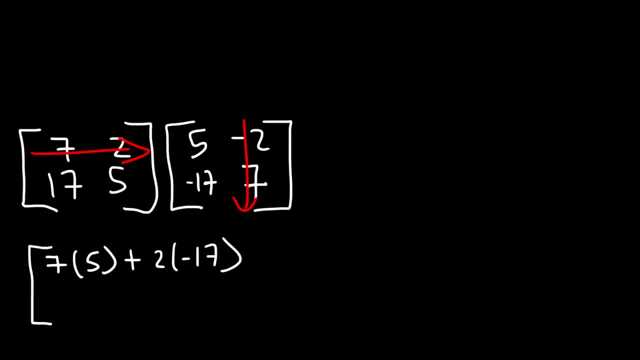 And then row one times column two. So that's going to be seven times negative two plus two times seven, And then it's going to be row two times column one. Okay, So that's seventeen times five and five times negative seventeen, And then finally row two times column two. 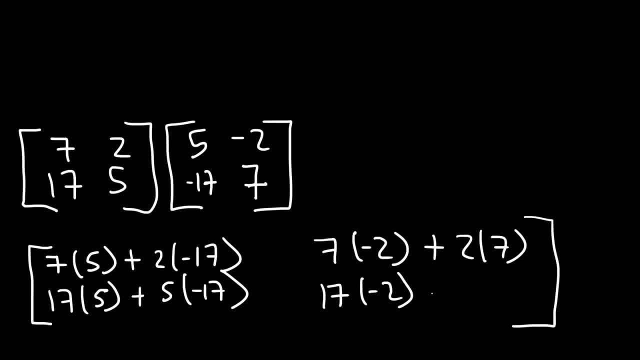 So that's going to be seventeen times negative. two plus five times seven. So now let's simplify: Seven times five is thirty-five. Two times negative seventeen, that's negative thirty-four. Seven times negative. two is negative fourteen. Two times seven is fourteen. 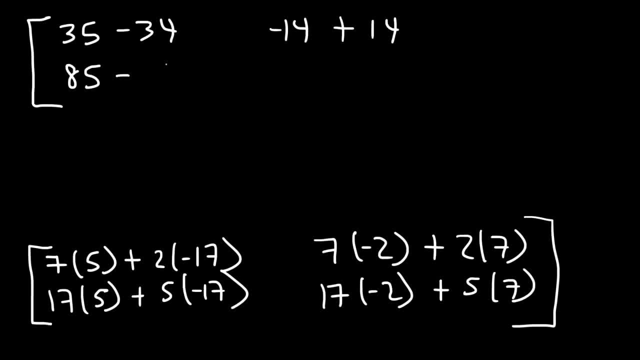 Seventeen times five is eighty-five And five times negative. seventeen is negative eighty-five, And here we're going to have negative thirty-four plus thirty-five. So these two, they completely cancel. Thirty-five minus thirty-four is one Negative. fourteen plus fourteen. 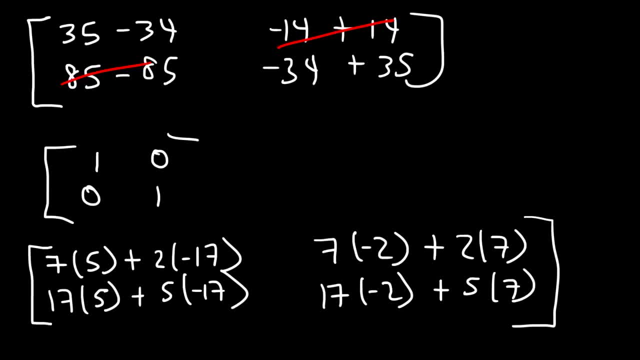 That's zero. Eighty-five minus eighty-five is zero, And this is one as well. So we do get the multiplicative identity matrix, Which means that the inverse that we had A negative one, that was indeed the inverse of matrix A. 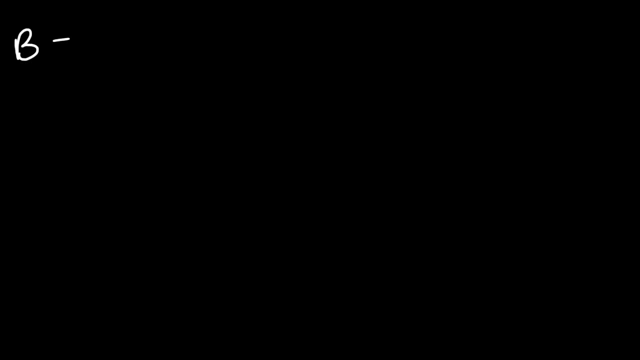 Now it's your turn. So let's say, if we have matrix B and it's still a two-by-two matrix, Let's say it's eight, six, five and four. Determine the inverse. Determine the inverse. Determine the inverse of matrix B And then show that those two are definitely inverses. 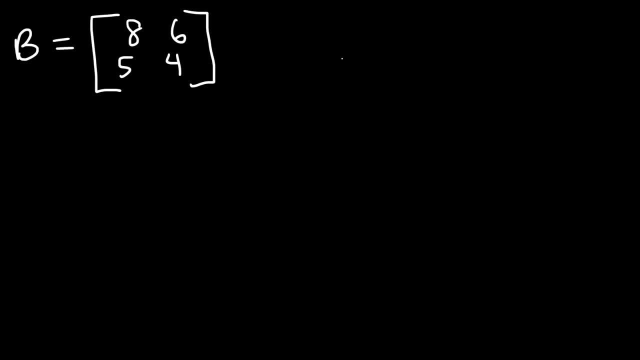 of each other. So first we need to realize that A is equal to eight, B is equal to six, C is five, D is four, And let's write the formula. So the inverse of matrix B is going to be one over A D minus B, C, And then we're going. 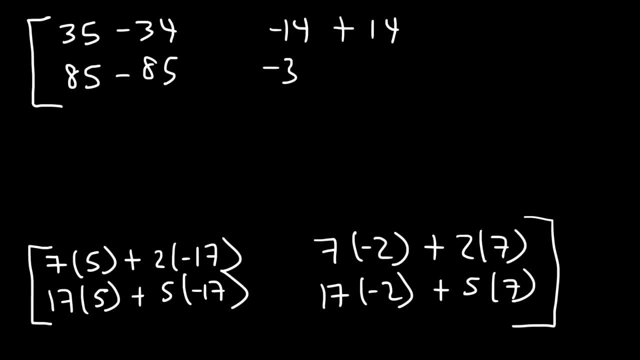 times negative. 17 is negative 85, and here we're going to have negative 34 plus 35. so these two they completely cancel. 35 minus 34 is 1. negative 14 plus 14 at 0, 85 minus 85, 0, and this is 1 as well. so we do get the multiplicative. 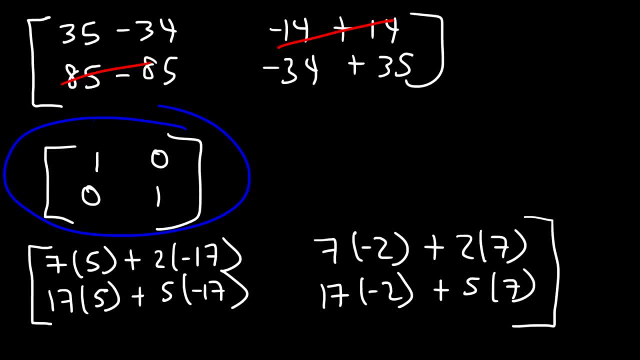 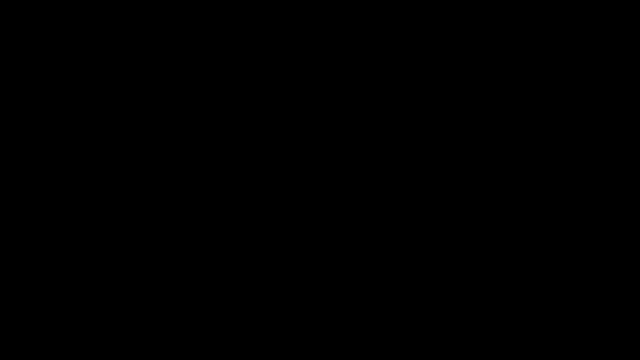 identity matrix, which means that the inverse that we had a negative 1, that was indeed the inverse of matrix a. now what's your turn? so let's say, if we have matrix B and it's still a 2 by 2 matrix, let's say it's 8, 6, 5 and 4, determine the inverse of matrix B and then show that those two 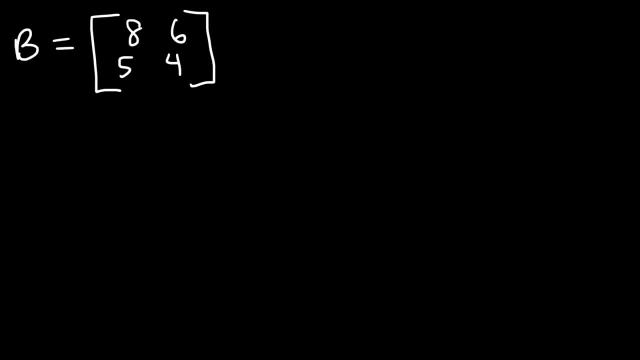 are definitely inverses of each other. so first we need to realize that a is equal to 8, B is equal to 6, C is 5, D is 4, and let's write the formula. so the inverse of matrix B is going to be 1 over A, D minus BC, and then we're. 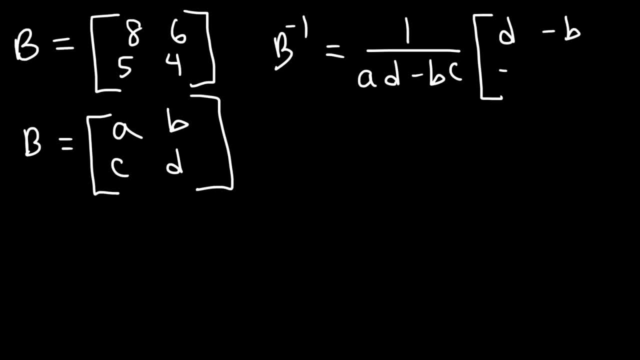 going to have the elements D, negative, B, negative c and a. so in this example, a is 8, D is for, B is 6, C is 5. so D said it's 4 negative, B is negative, 6, C is negative, 5 and a is 8. now, 8 times 4 is 32 and 6 times 5 is 30. 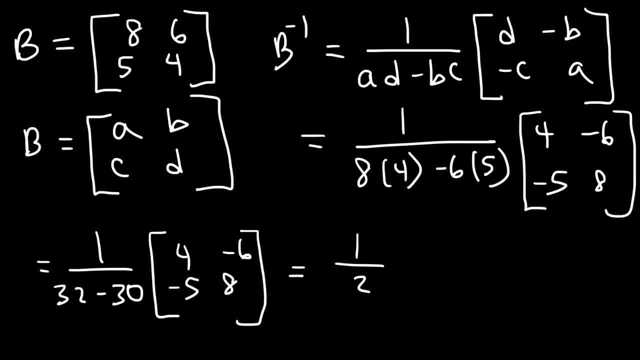 and 32 minus 30 is 2. so we have 1 half of 4 negative, 6, negative 5 and 8. so now we need to distribute. the 1 half half of 4 is 2, half of negative 6 is negative 3. 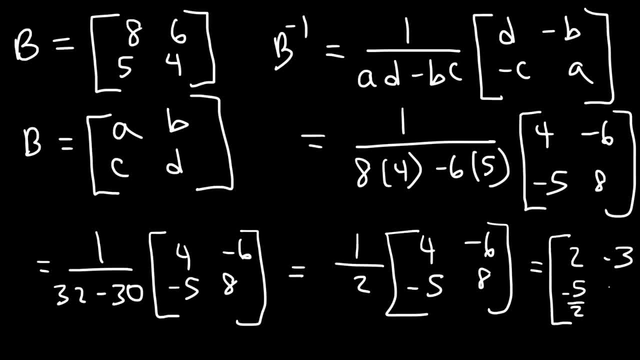 and then we're gonna have a negative 5 over 2 and half of 8 is 4. so that's the inverse of B, which I'm going to rewrite it at the top. so the inverse of matrix B is 2 negative, 3 negative, 5 over 2 and 4. 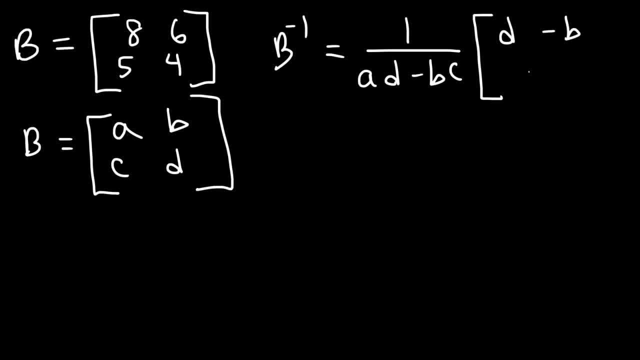 to have the elements D, negative B, negative C and A. So in this example A is eight, D is four, B is six, C is five. So D, we said, is four, Negative B is negative six. Negative C is negative five. 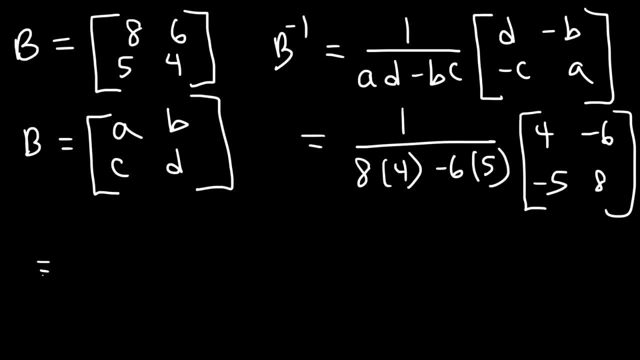 And A is eight. Now, eight times four is thirty-two, And six times four is thirty-two, And six times five is thirty, And thirty-two minus thirty is two. So we have one half of four negative, six negative five and eight. 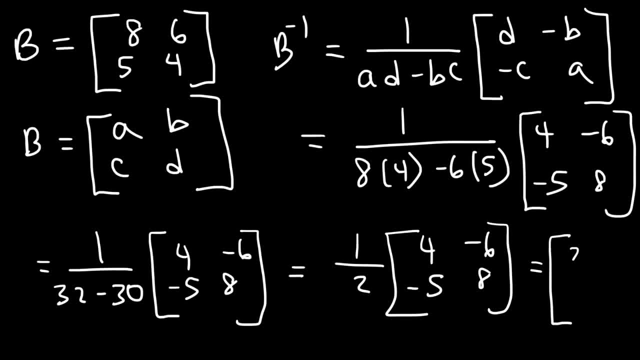 So now we need to distribute the one half. Half of four is two, Half of negative six is negative three, And then we're going to have negative five over two, And half of eight is four. So that's the inverse of B, which I'm going to rewrite it at the top. 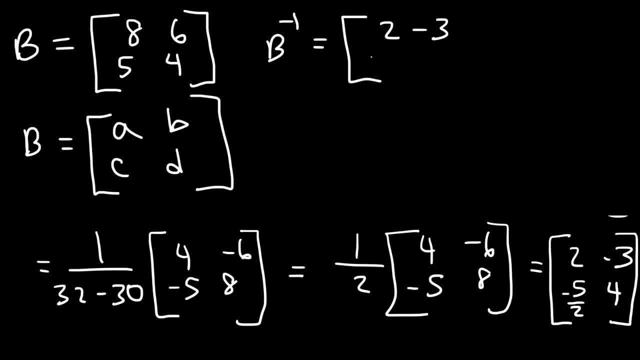 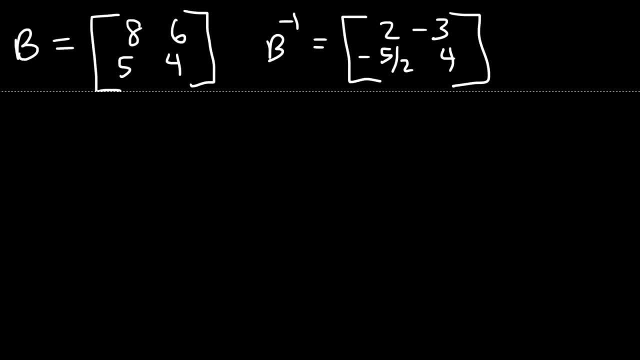 So the inverse of matrix B is two negative, three negative, five over two and four. Now go ahead and confirm that B times the inverse of B is going to equal to the multiplicative identity matrix one, zero, zero, one. Go ahead and show that. 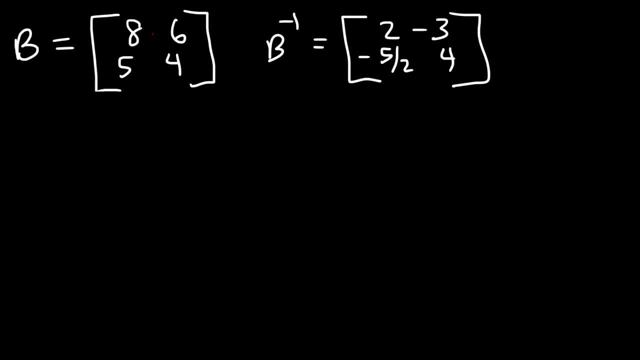 So let's multiply the two matrices. So row one times column one. Let's write it out: So it's going to be eight times two plus six times negative five over two. Next we have row one. It's going to be row two times column two. 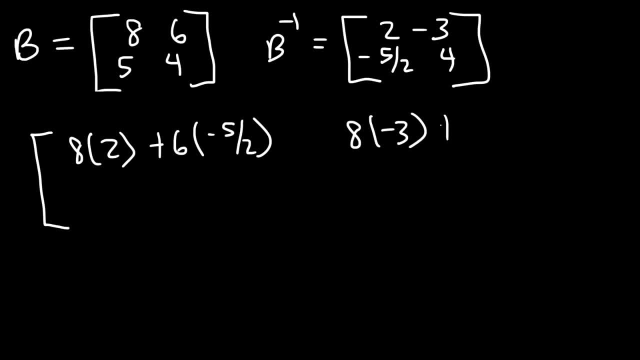 And then that's going to be eight times negative, three plus six times four, And then it's going to be row two times column one, So that's five times two plus four times negative, five over two, And then row two times column two. 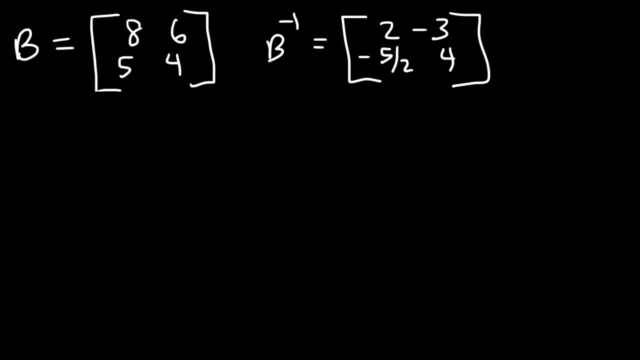 now go ahead and confirm that B times the inverse of B is going to equal to the multiplicative identity matrix 1 0 0- 1. go ahead and show that. so let's multiply the two matrices. so row 1 times column 1. let's write it out. 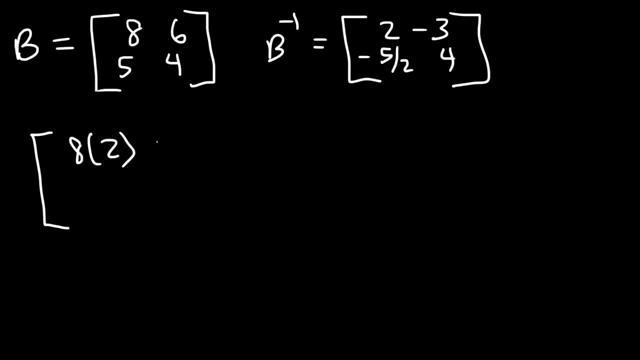 so it's going to be 8 times 2 plus 6 times negative 5 over 2. next we have row 1 times column 2, and then that's going to be 8 times negative 3 plus 6 times 4, and then it's going to be row 2 times column 1. 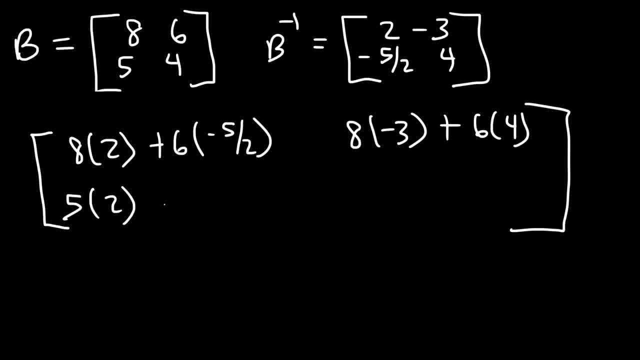 so that's 5 times 2 plus 4 times negative, 5 over 2, and then row 2 times column 2, so it's going to be 5 times negative, 3 plus 4 times 4, now 8 times 2. 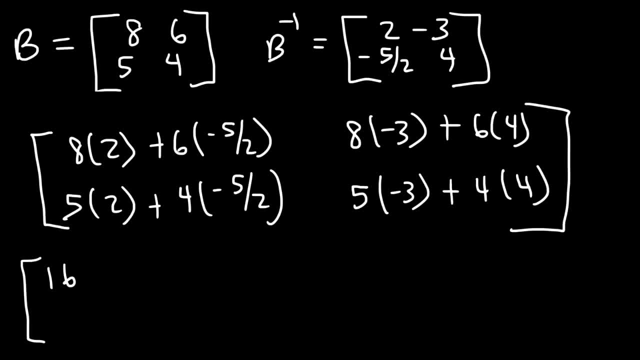 is 16. what 6 times negative? 5 over 2. 6 divided by 2 is 3- 3 times negative: 5. it's negative 15, 8 times negative. 3 is negative: 24, 6 times 4 is 24, 5 times 2 is 10. 4 divided by 2 is 2 times negative 5. 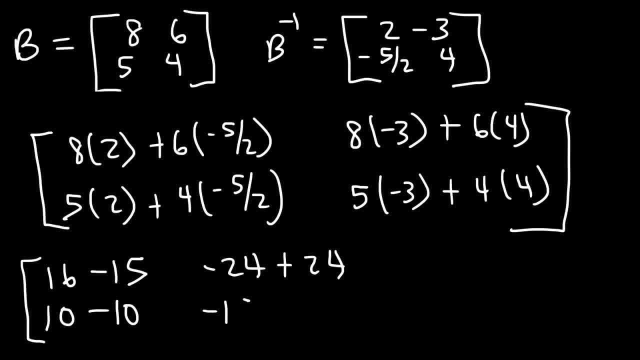 that's negative 10, 5 times negative. 3 is negative 15. 4 times 4 is 16. then there's 3 times negative, 5 times negative: 14. this gives me square root 3 times. I took around 4 times plus 4 times 4, then we have 25. so we have to have: 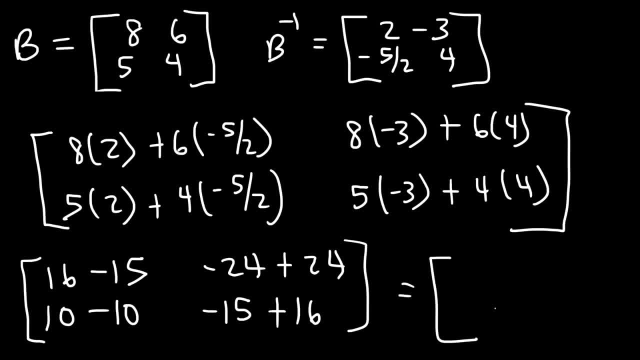 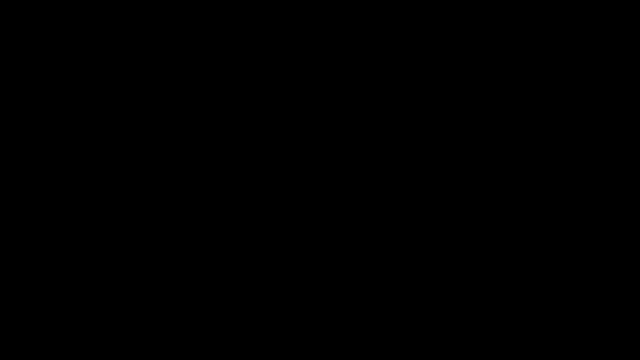 Now, 16-15 is 1, negative, 24 plus 24 is 0,, 10-10 is 0, and negative 15 plus 16 is 1.. So, as you can see, we do get the identity matrix.